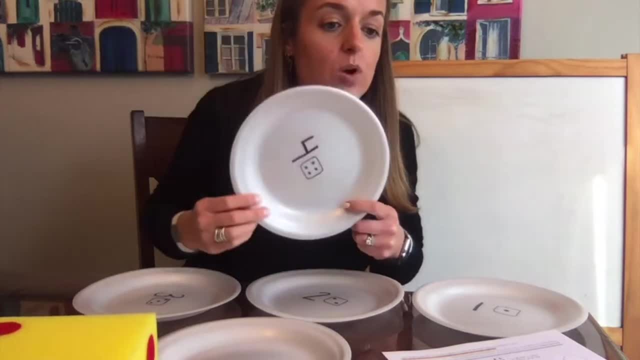 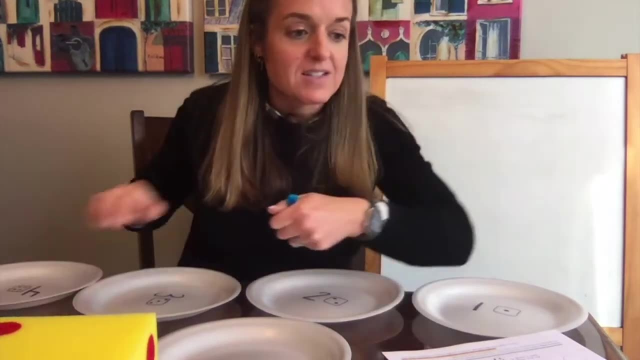 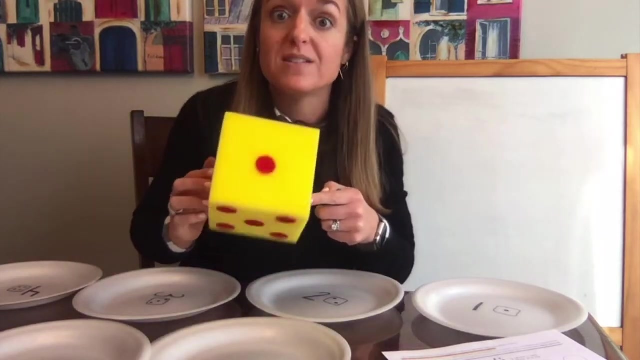 on a four, then we're going to put a blueberry on the four, the number four pancake. okay, Our die has six sides, so each of our six pancakes has an even chance of getting a blueberry. It has a one in six chance of getting a blueberry, right? So why don't we find out what happens when we roll? 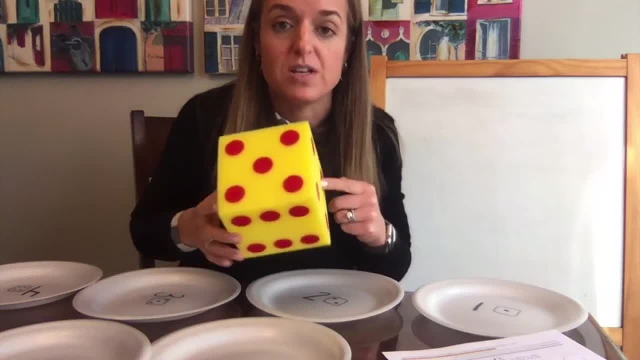 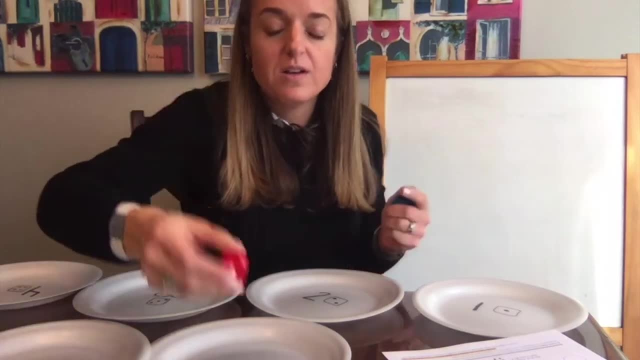 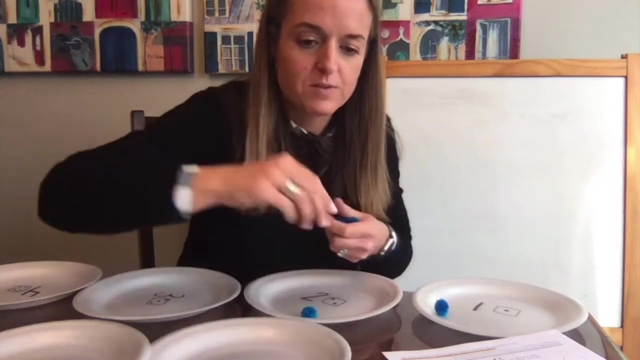 this die 15 times and see what the distribution is. So I love this big die to use in class. I found these on Amazon For right now for my video, I'm going to use a little one because I don't quite have the space for such a big, giant one. So that time I got a one, two, two, one, three. 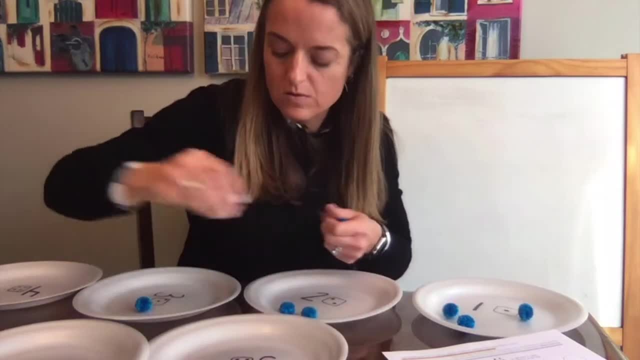 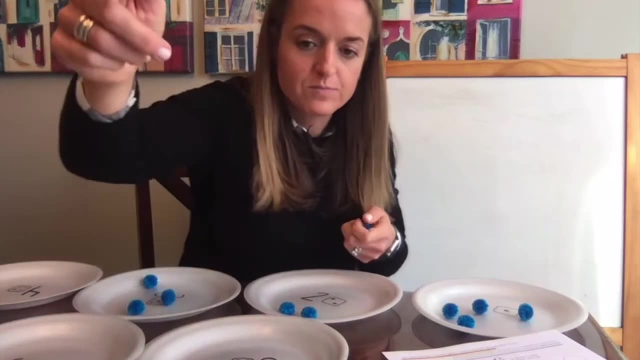 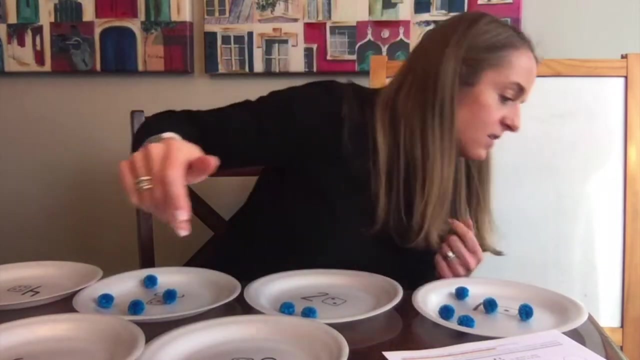 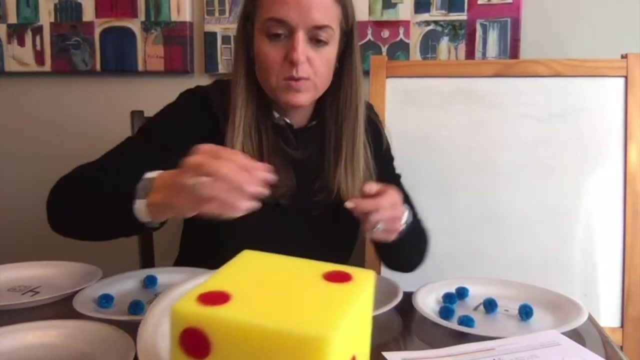 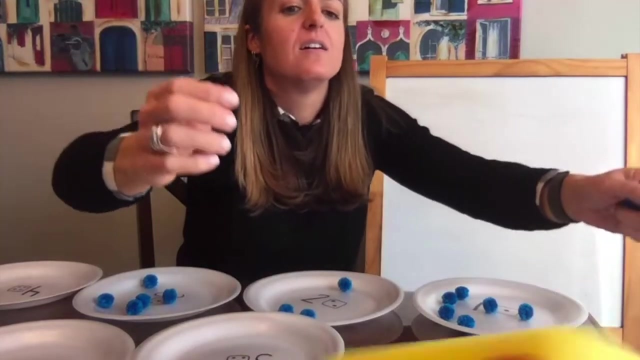 one, three, one, three, three, one. Oh, my goodness Going to the floor. One, No, let's use our big one, since I lost that. one, Two, three, My goodness, Six. I got a six, Excellent. 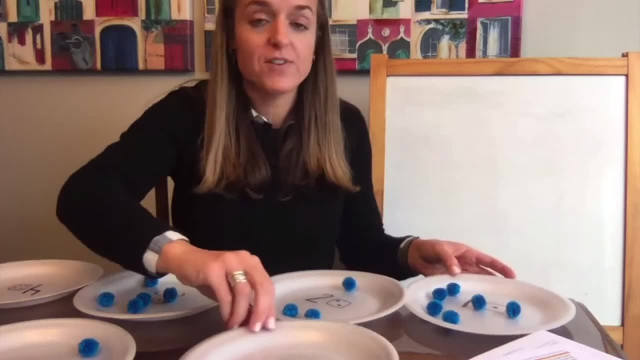 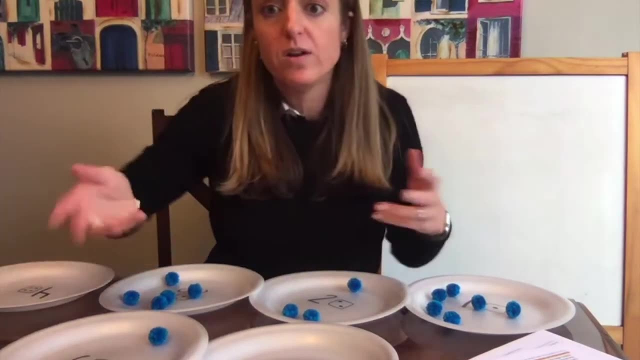 So now I did my, I distributed my 15 blueberries, and, man, it was really heavy on the one, two and three, wasn't it? I got a one on number six, but number four has none and number five has none. 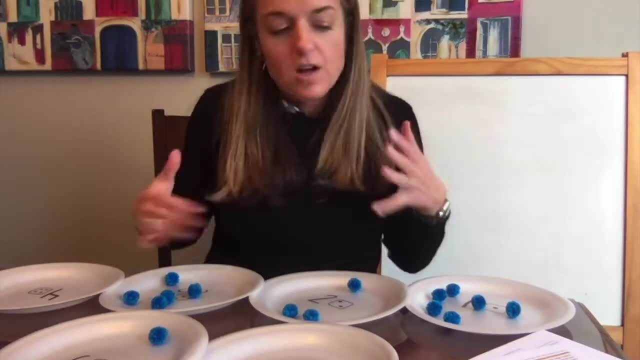 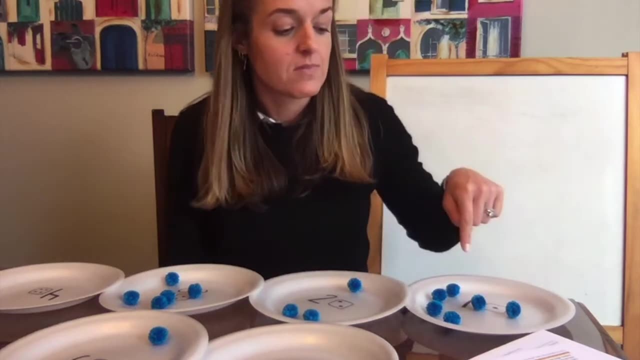 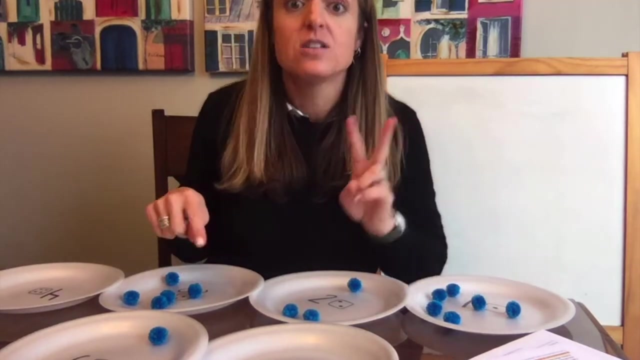 You'll probably get different results when you try it, but let's just talk about our results. How many pancakes got at least four blueberries? This one has at least four. This one has at least four. This one has five. This one has six. So two of them have at least two blueberries. How many have less than two? 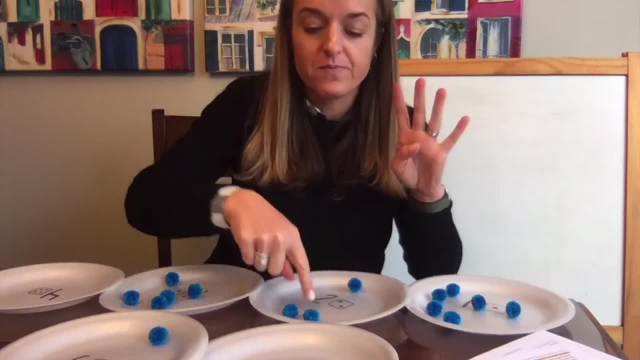 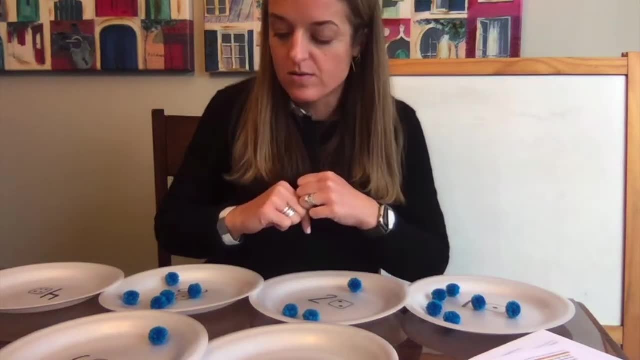 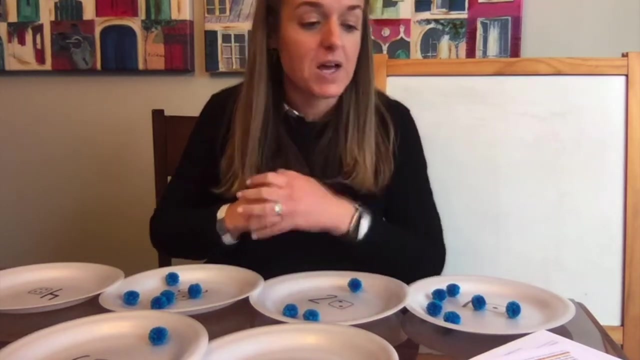 I mean sorry. how many have less than four? One, two, three, four, Four of them have less than four. How many pancakes got more than four? Two got more than four. How many got exactly four? None, None of them got exactly four. Are there any outliers, meaning results that don't seem to fit the 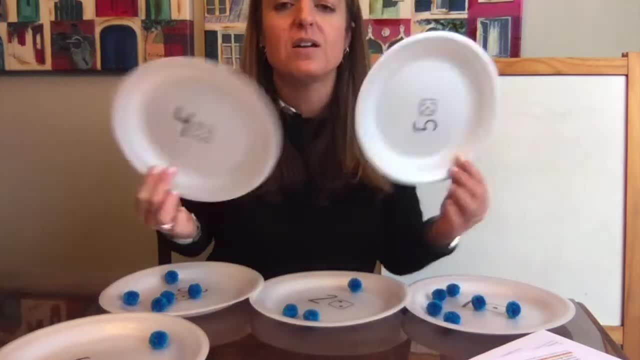 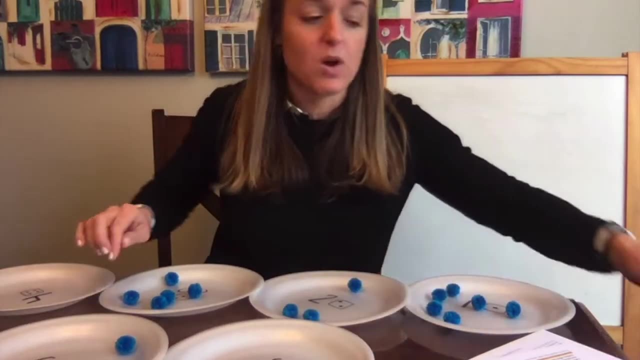 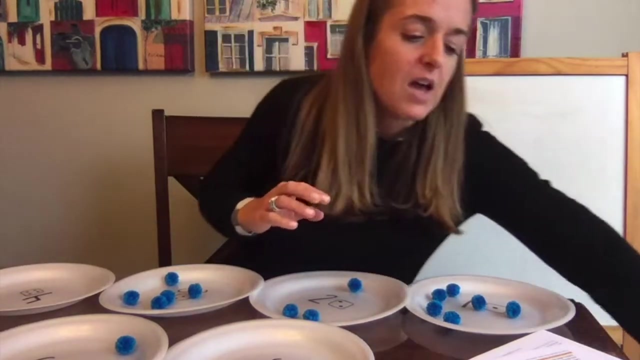 normal pattern, Wouldn't you say these are outliers with zero. Does zero seem like? I mean, was that surprising? Did you expect it to be zero, to get zero when there was an even chance on the die of getting one out of six, chance of getting all the numbers? Yeah, I feel like those were. 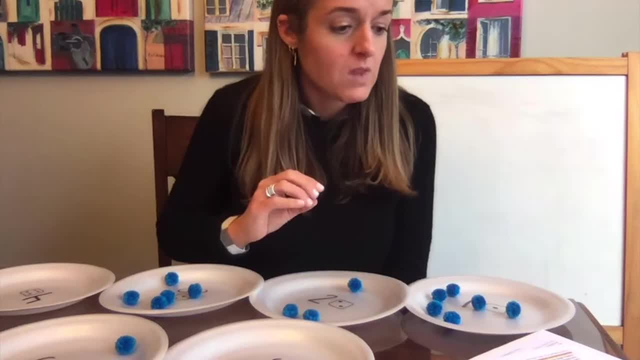 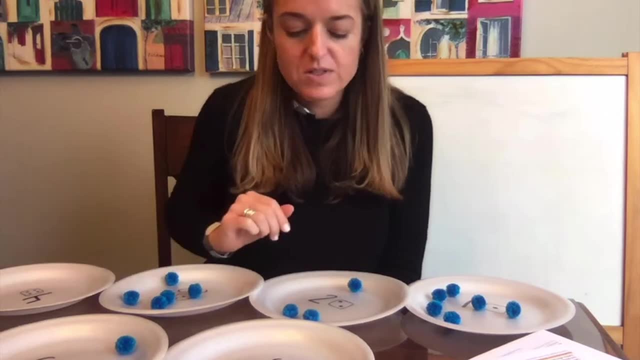 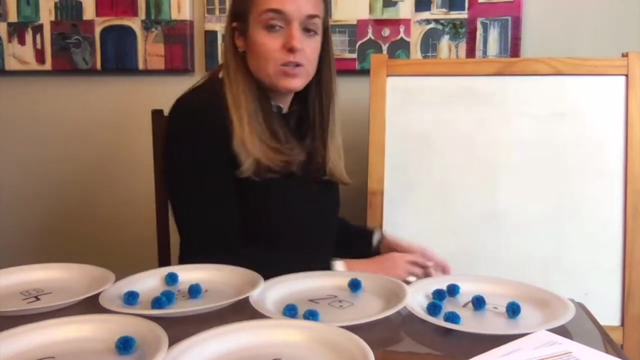 probably outliers. What do you think the chances are of getting four blueberries on one pancake? then, Based on our results here, what are our, what is our chance of getting at least four blueberries on one pancake? So back to our, back to our probability equation. we have our, 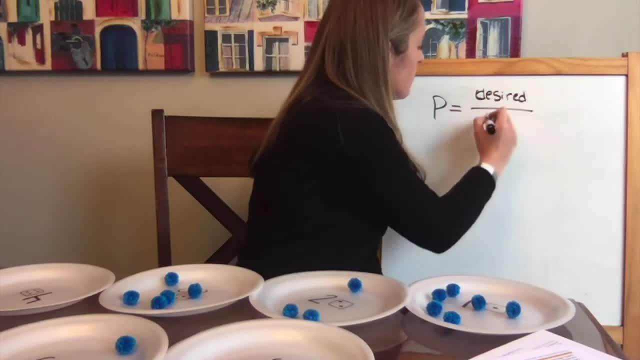 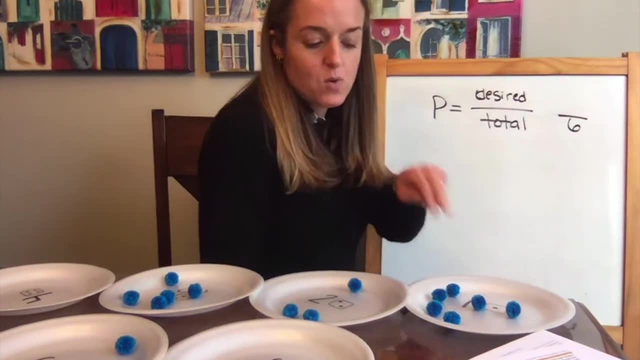 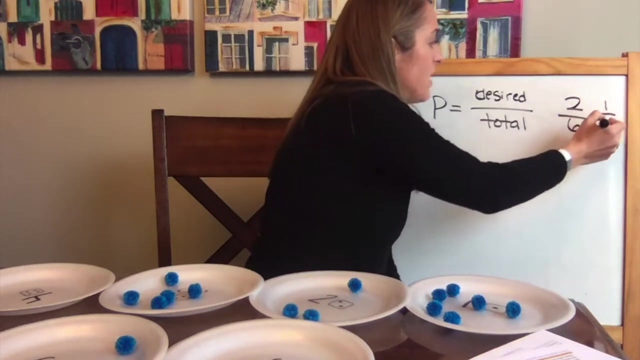 desired outcomes over our total outcomes. So if we have six pancakes, then how many of them will have at least four? We think two. Based on our results, we think two And big kids. if we reduce that one out of three chances, or 33% chance of getting at least four. 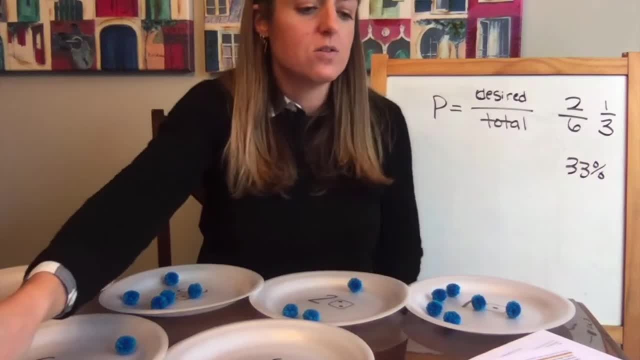 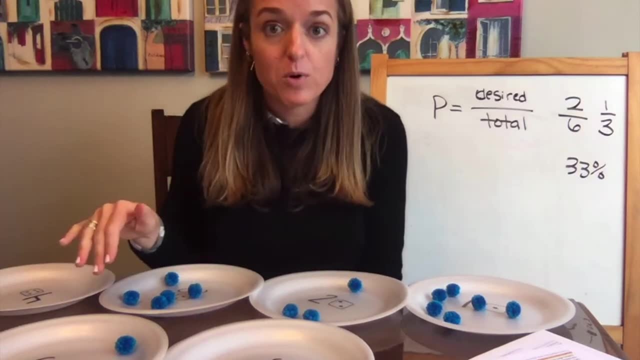 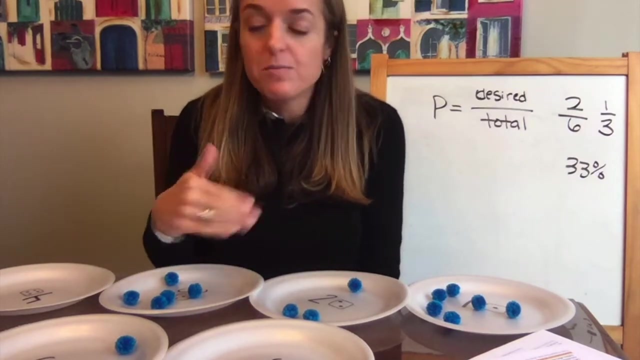 blueberries in a pancake. Those are not super high odds. We could keep going with this by doing 15 more rolls and adding 15 more blueberries and see if that changes anything. So that's what I recommend you do now: Grab your die again, roll 15 more, add your blueberries and see if it changes. 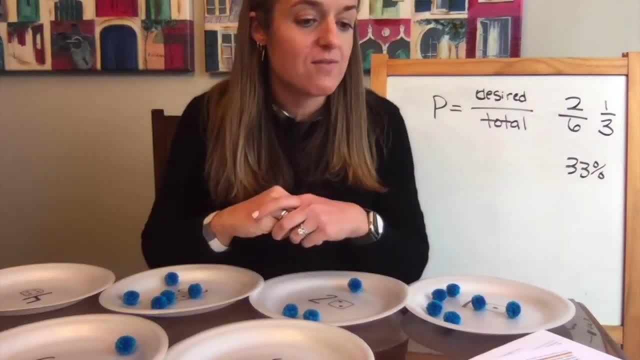 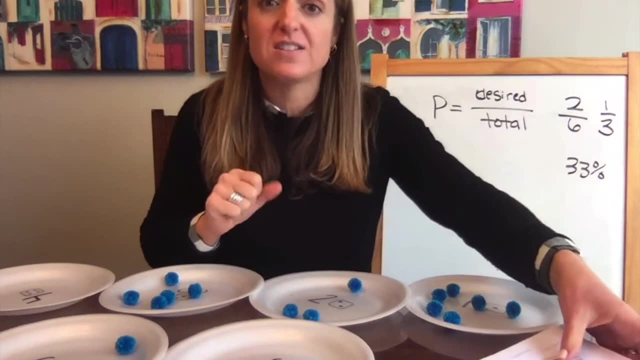 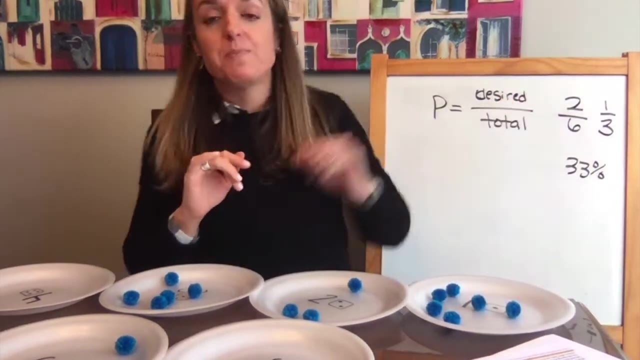 your results And ask these same questions again. How many have more than four, then? And see what happens to your, to the probability and to the chances of getting pancakes that have at least four blueberries. That's what we're looking for. Our desired outcome is pancakes with at least 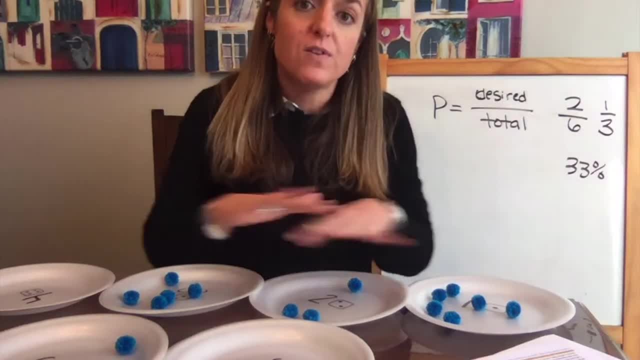 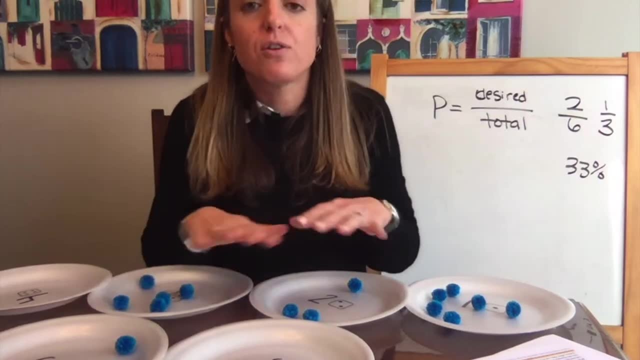 four blueberries. So we did. we started with 15 rolls and 15 blueberries and then now we're going to go for 30. So we're going to do 15 more. So we have a total of 30 blueberries. 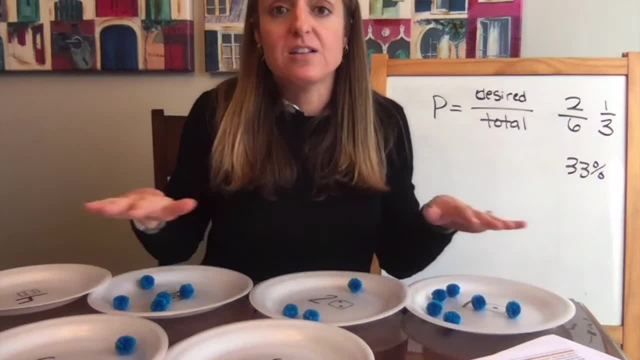 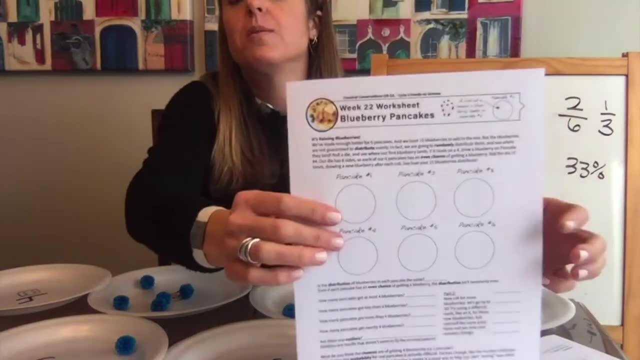 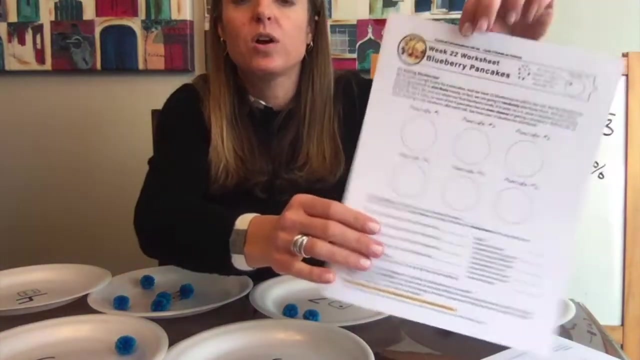 15 rolls with that die And you guys can do that as a class all the way to 30. Or you could do 15 as a class And then you can pass out this wonderful worksheet from Nicole Liam Yang's worksheet that's on CC Connected, And kids can work either individually or in pairs. I think pairs would be. 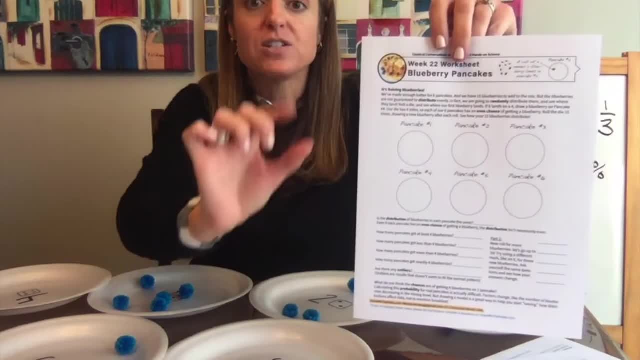 good to do this all from the from scratch, from one roll all the way to 15 and just draw little blueberries on their blueberries for 30. And then you can do that as a class all the way to 30. And